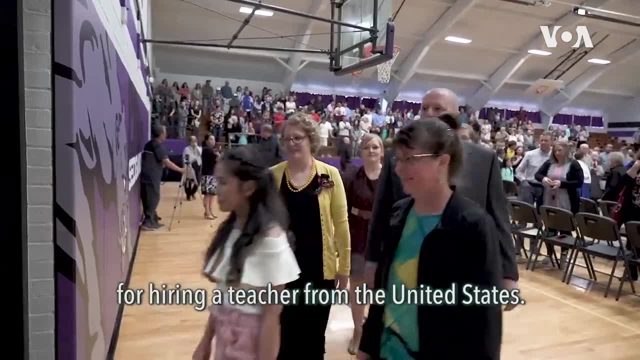 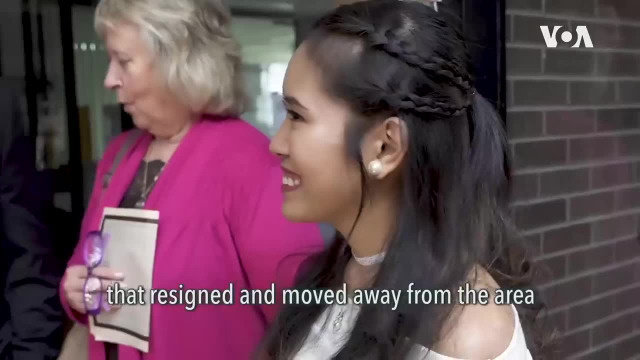 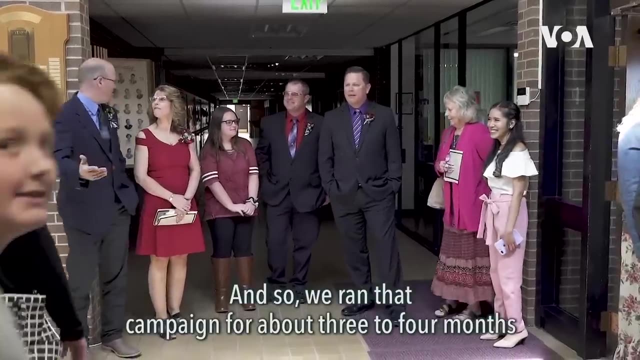 options for hiring a teacher from the United States. Two years ago I had a long time math teacher that resigned and moved away from the area that had been with our district for about the last 12 years And so we ran that campaign for about three to four months trying. 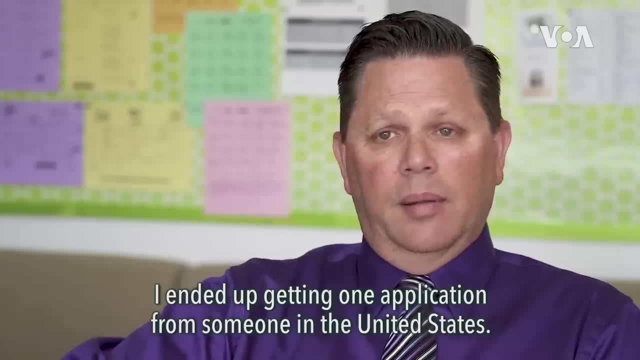 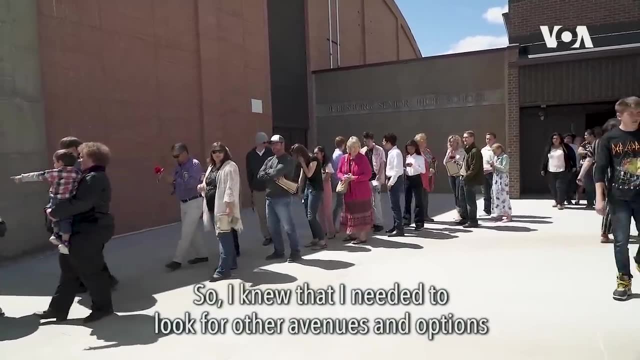 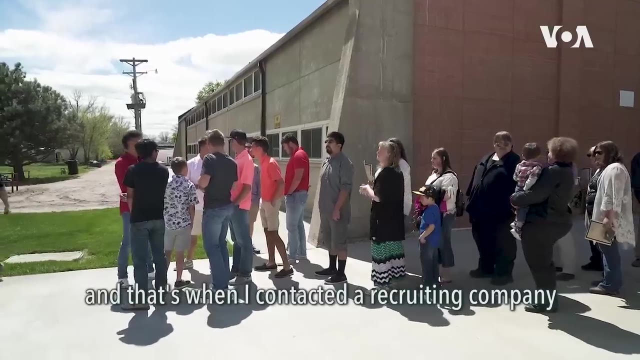 to recruit and get applicants to fill that position. I ended up getting one application from someone in the United States. I wasn't able to recruit the one application that I had, So I knew that I needed to look for other avenues and options, and that's when I contacted a recruiting. 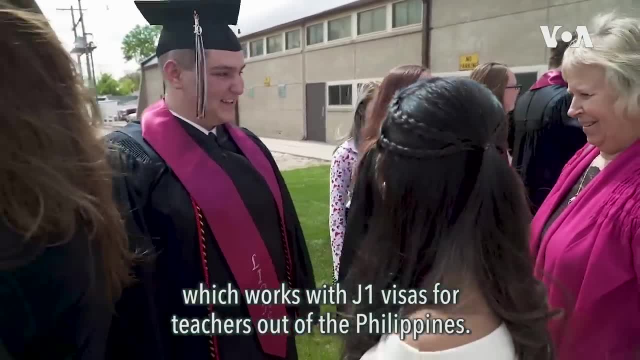 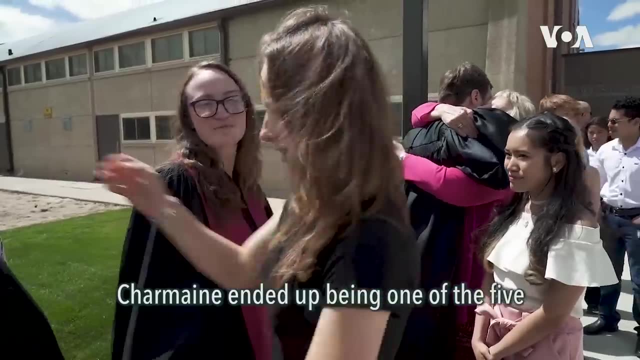 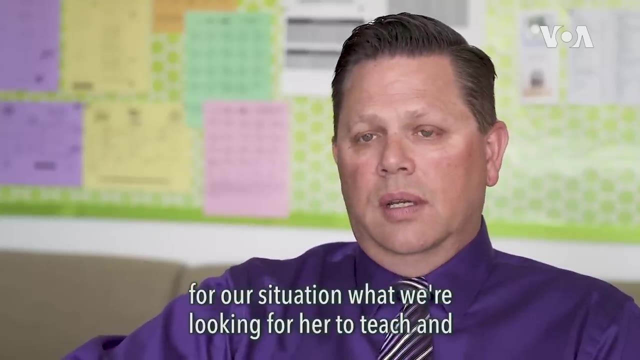 company which works with J-1 visas For teachers out of the Philippines. I did five interviews using video conferencing and Charmaine ended up being one of the five that we felt like was the best fit for our situation, what we're looking for her to teach and work in a small school district. 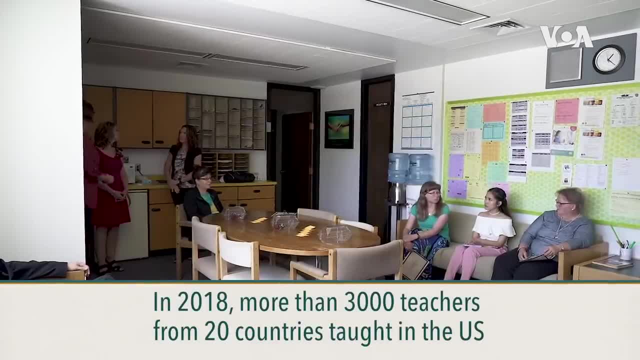 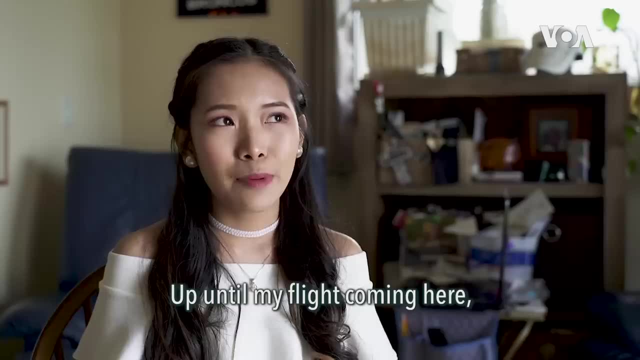 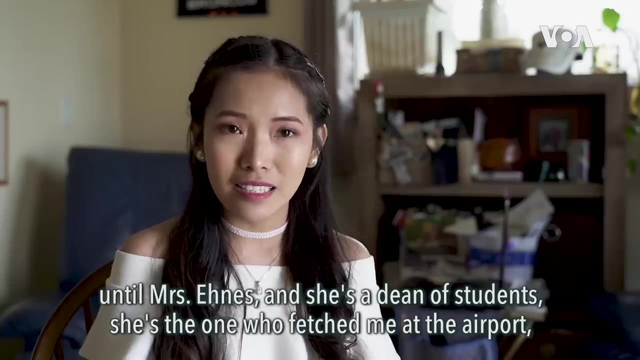 First I couldn't believe it and I was thinking it could be a scam, Up until my flight coming here. I'm still not believing it, Until Mrs Ines- and she's a dean of students- she's the one who fetched me at the airport. That was the time that I said: okay, this. 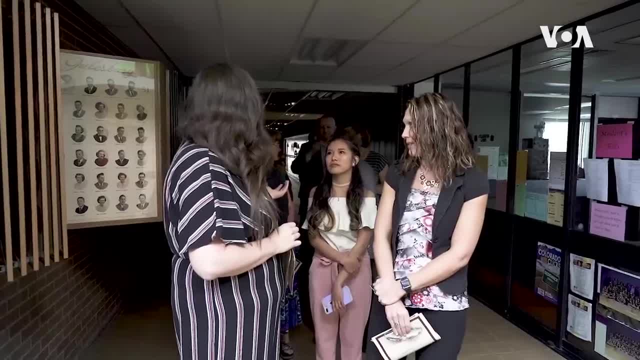 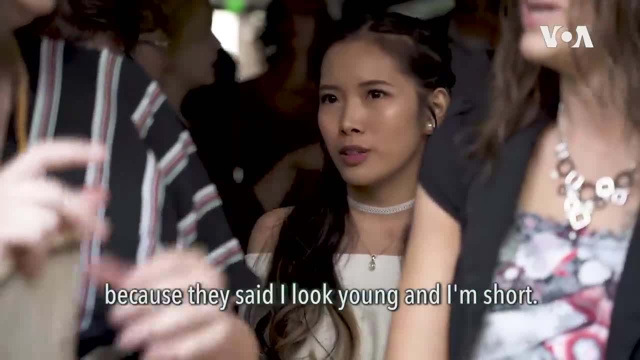 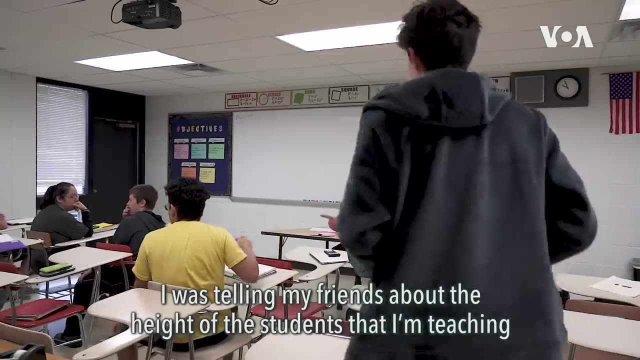 is real because they're actually here. First they thought that I'm also a student because they said: I look young and I'm short. I'm just a fellow student, like a foreign exchange student, And they are huge. I was telling my friends about it. I was telling my friends about it. I was telling my friends. 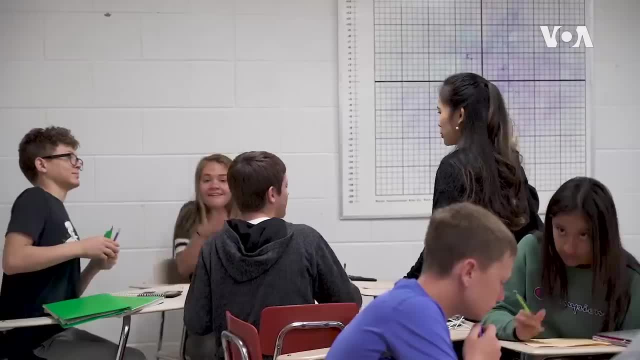 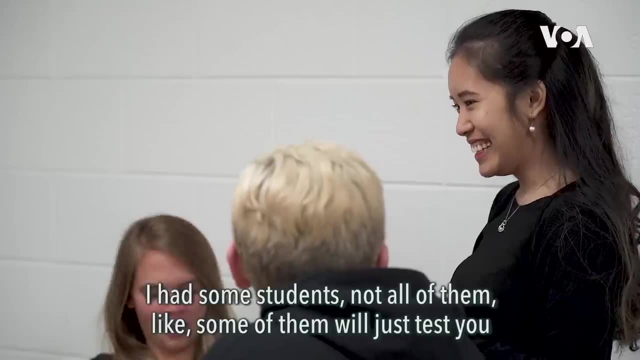 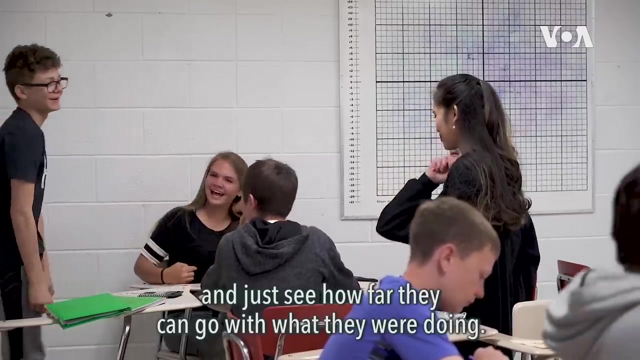 about it. I was telling my friends about the height of the students that I'm teaching and they all get shocked. I've had some challenges. during my first year I had some students- not all of them- like some of them will just test you and just see how far they can go with what they were doing. 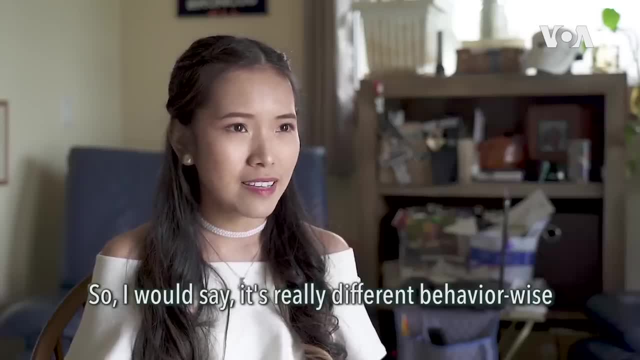 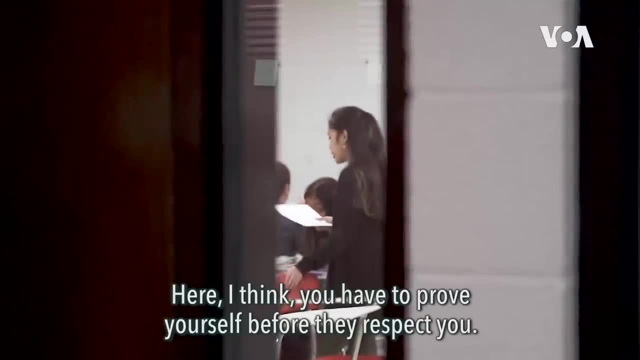 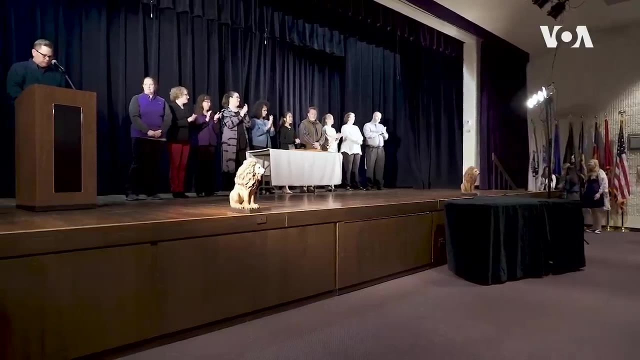 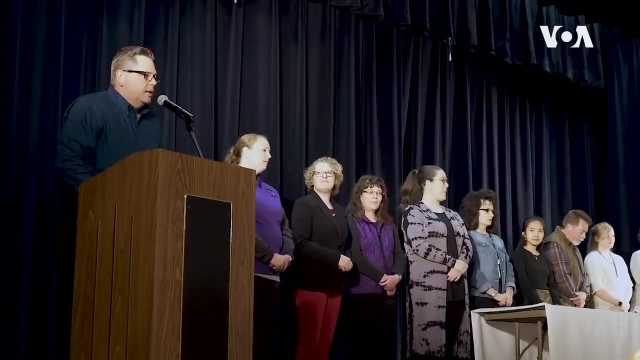 So I would say it's really different behavior-wise, because in the Philippines you don't have to do anything. They see you in uniform as a teacher. They respect you. Here, I think you have to prove yourself before they respect you. The NWEA High Growth Award in Mathematics and Science. Nice job, 8th grade, You guys. 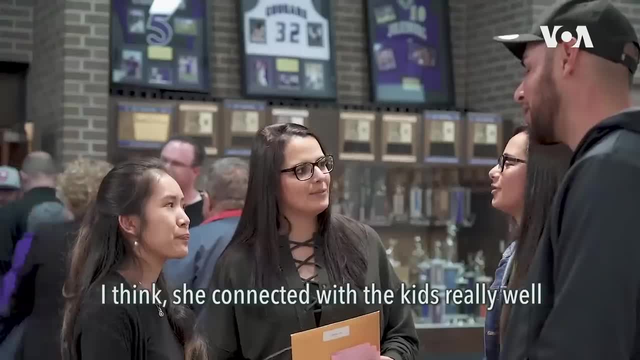 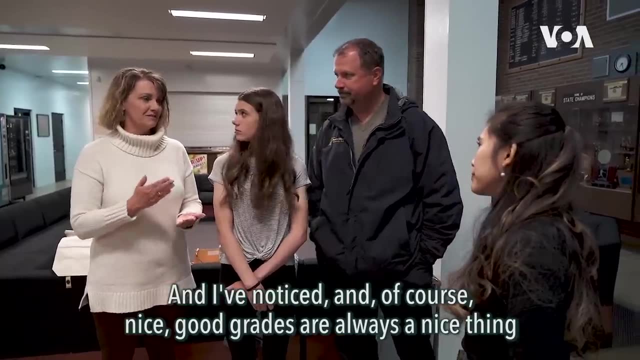 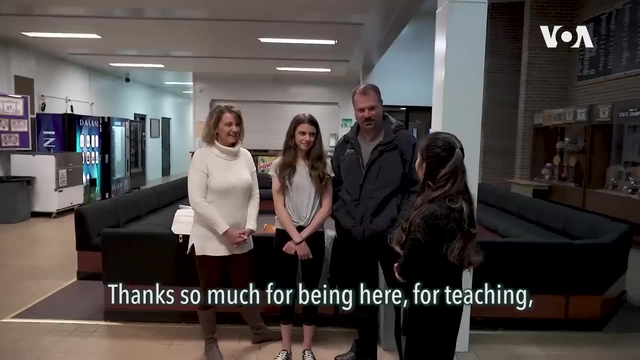 have a lot of promise in both. I think she connected with the kids really well and she's a very good mathematics teacher. What I've noticed- and of course, good grades are always a nice thing, but just her confidence And that she's able to come home and do it by herself. 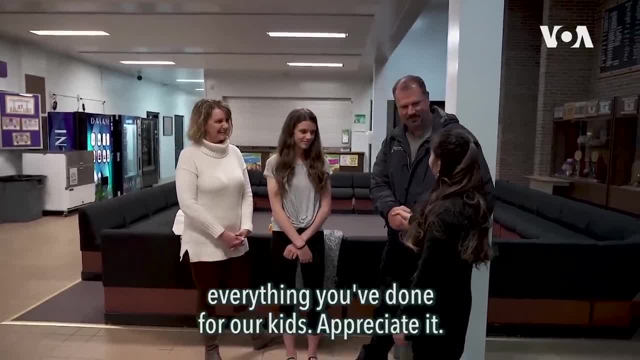 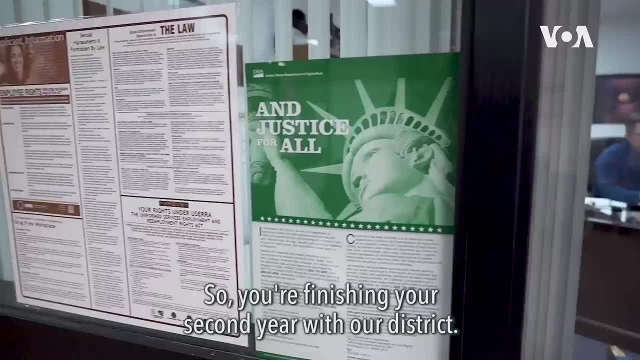 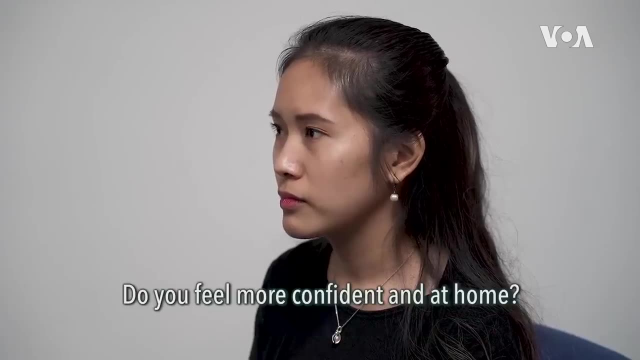 Thanks so much for being here. I appreciate everything you've done for our kids. Thank you, And have a wonderful summer. So you're finishing your second year with our district, And so did the second year go a little better than the first year. Do you feel more confident and at home? 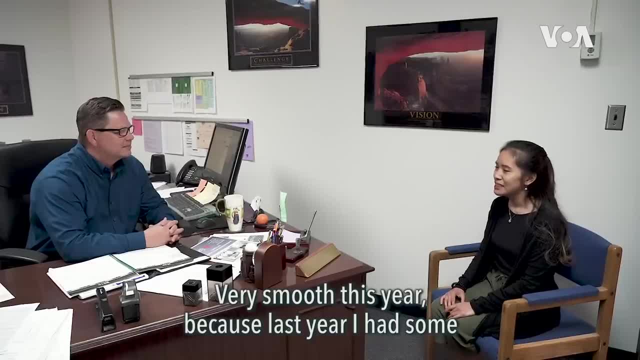 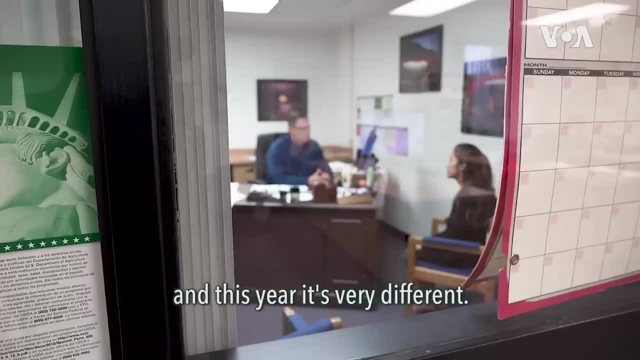 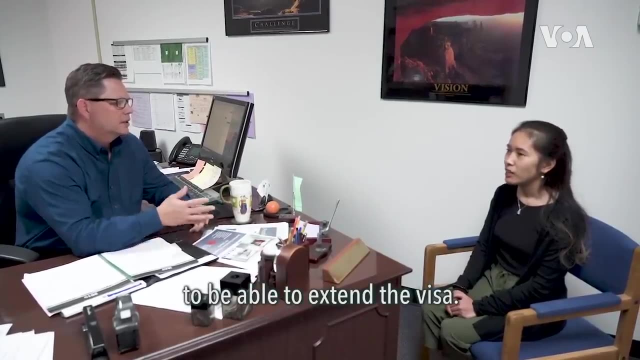 Very smooth this year Because last year I had some classroom management issues with some of the students, The kids, And this year it's very different. We want to stay Okay And do you know what that process looks like to be able to extend the visa? 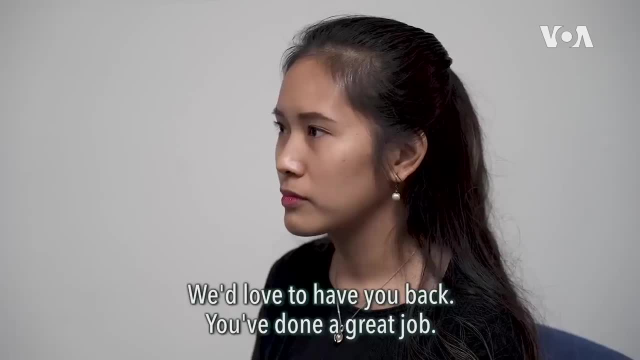 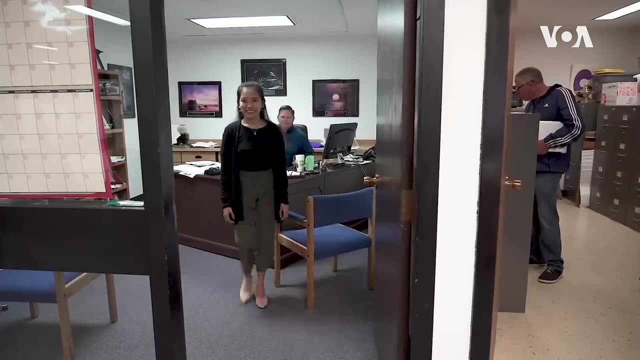 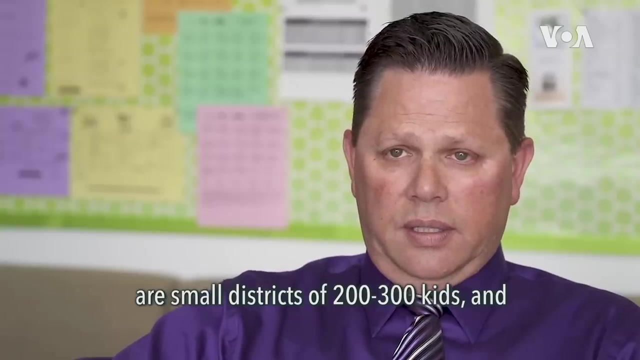 No, I will probably do some research about it. We'd love to have you back. You've done a great job, Thank you. Thank you very much. Thank you. All right, Have a good day You too. We're in an area here where all the school around us are small districts of two, three. 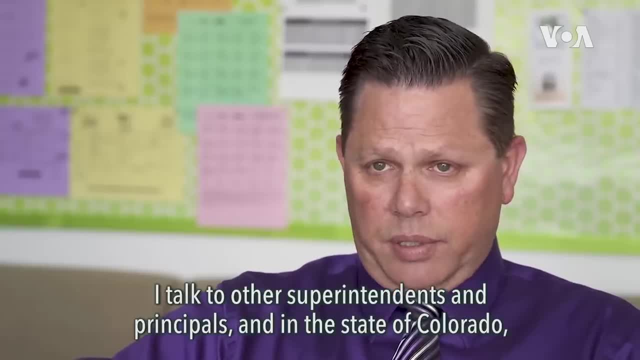 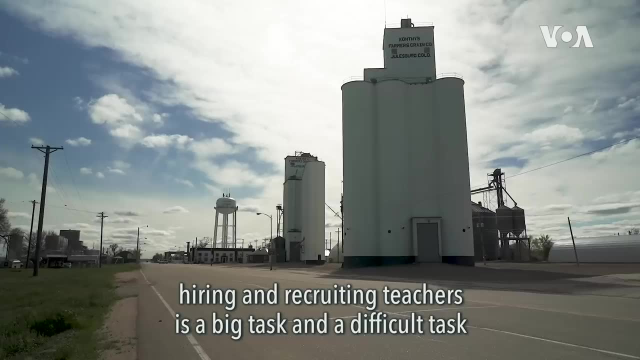 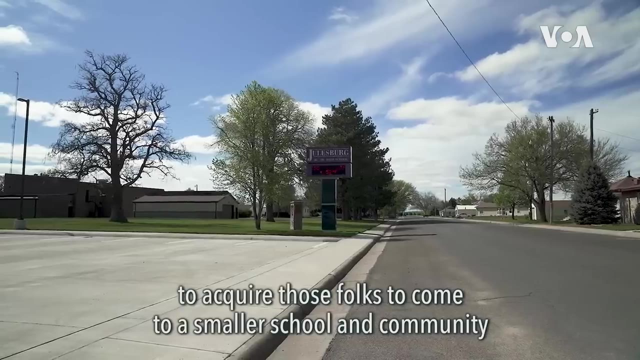 hundred kids- And I talk to other superintendents and principals- And in the state of Colorado even in our neighboring states, And hiring and recruiting teachers is a big task and a difficult task to acquire those folks to come to a smaller school and community, to 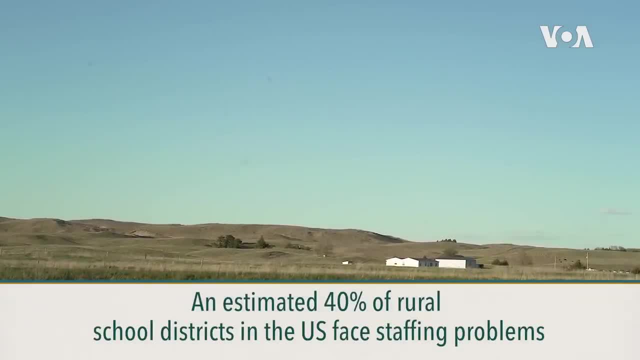 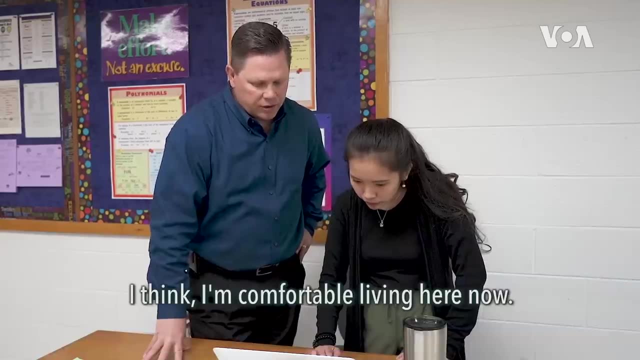 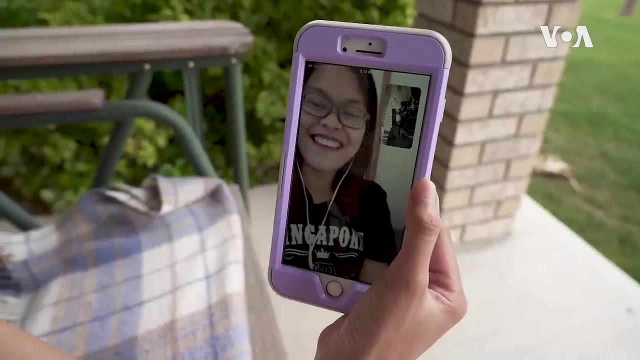 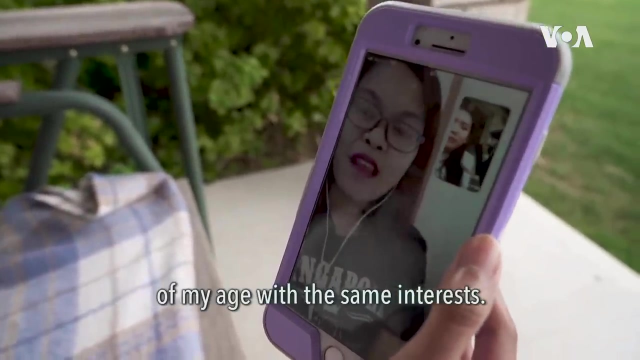 teach and live. Stand by. I think I'm close, I'm comfortable living here now, So I am planning to stay for as long as I could. She said she's shy. The challenges are: it's difficult to find friends of my age with the same interests. 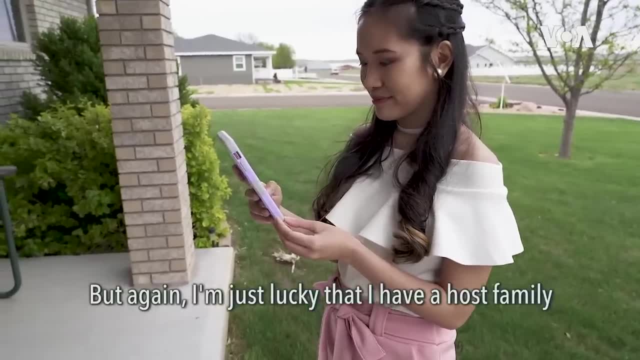 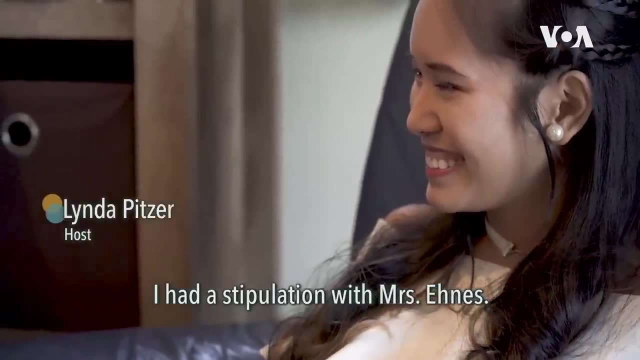 Bye-bye, But again, I'm just lucky that I have a host family with me who has been helping me. I had a stipulation with Mrs Enos. Did I ever tell you this? That you know if it. 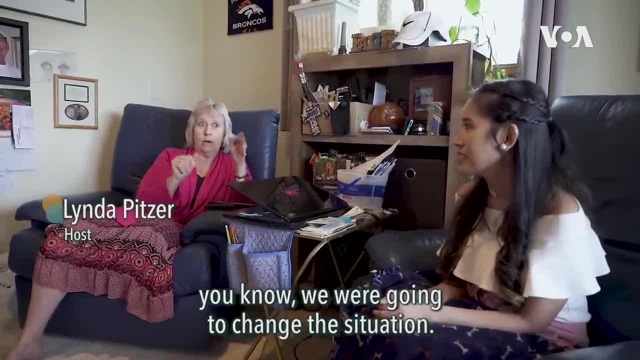 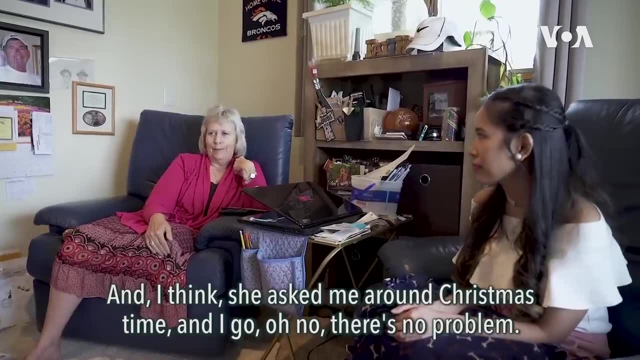 wasn't working out, I wouldn't be here. She said, you know, by Christmas time, you know we were going to change the situation And I think she asked me around Christmas time And I go: oh no, there's no problem.